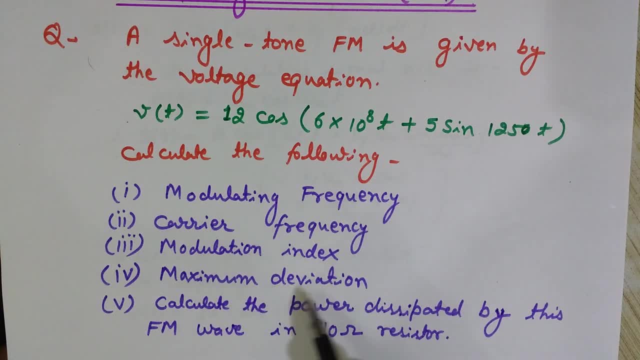 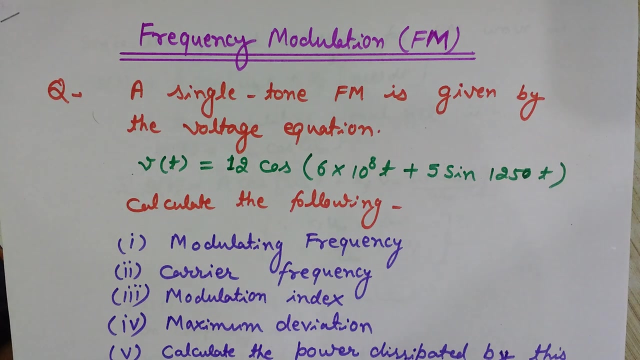 frequency modulation index, maximum deviation, and we'll also calculate the power dissipated by this fm wave in 10 ohm resistor. So keep watching this video till the end. Your many doubts will be cleared. So what we mean by frequency modulation? Actually, in frequency modulation, the frequency of the 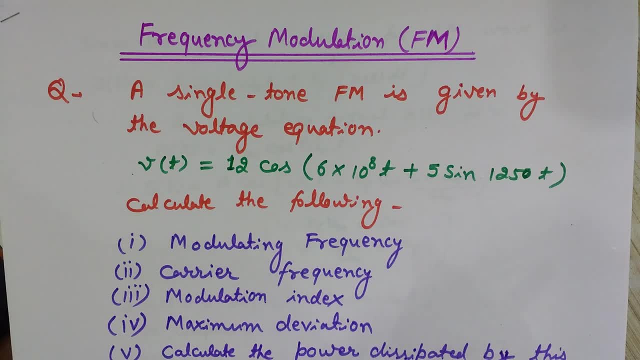 carrier wave is varied according to the instantaneous value of the modulating signal. Modulating signal is what It is: a message signal. So in this problem I have a single tone, fm. fm means frequency modulation, So a single tone, fm. Single tone means if the message signal 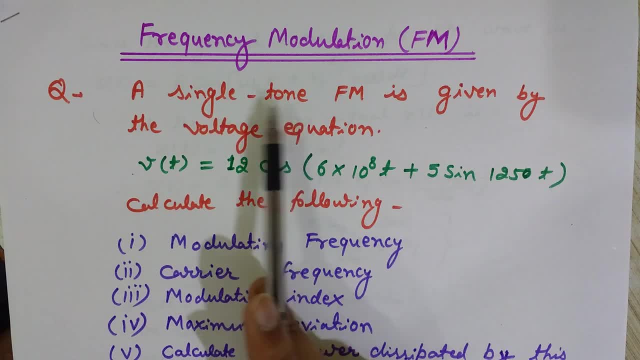 contains only a single frequency. Okay, So a single tone. fm is given by the voltage equation. This is the equation of this fm wave. 12 vt denotes the equation of fm. It is voltage, so it is vt. So 12 cos of 6 into 10. to the power, 8 t plus 5 sin, 1250 t. Okay, So I want to calculate these following: 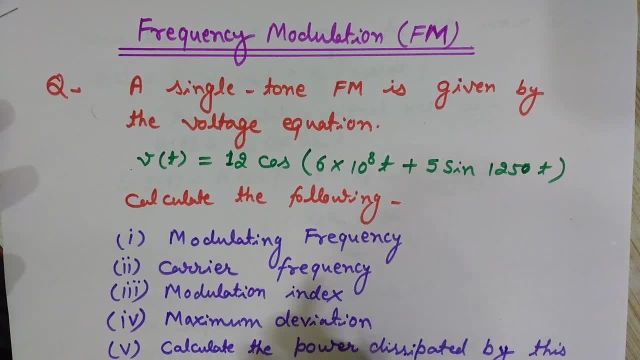 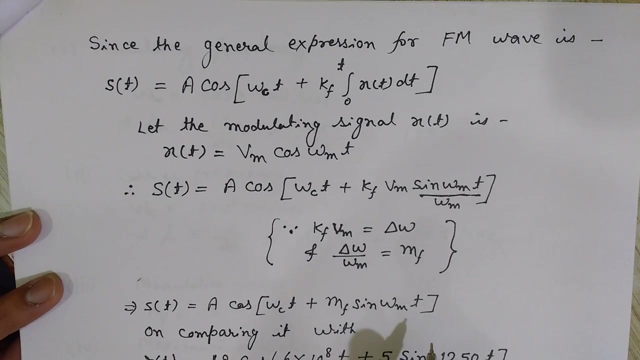 things. Now let's see how we do this. First of all, what will I do? I will convert this equation- given equation- into a general format of fm modulated wave. Then I will compare that equation with this given equation and will calculate all these things. Let's see how to do this, As we know that the general expression for the fm wave is: 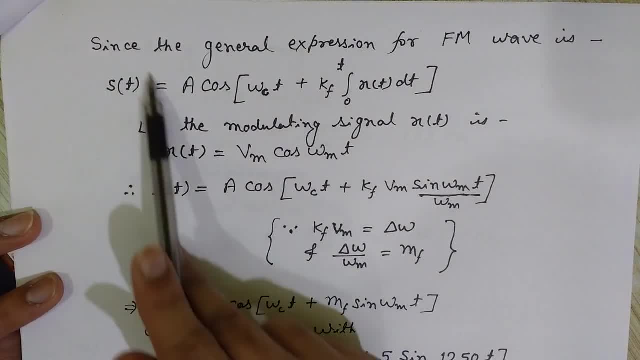 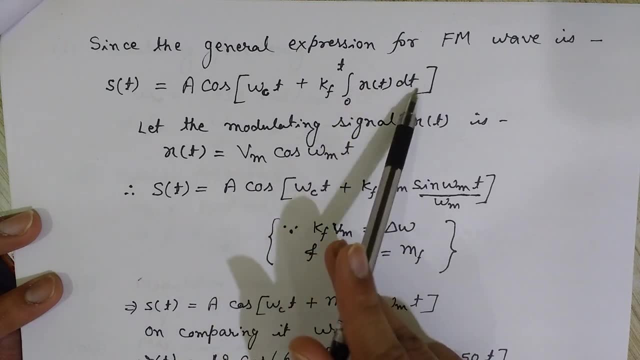 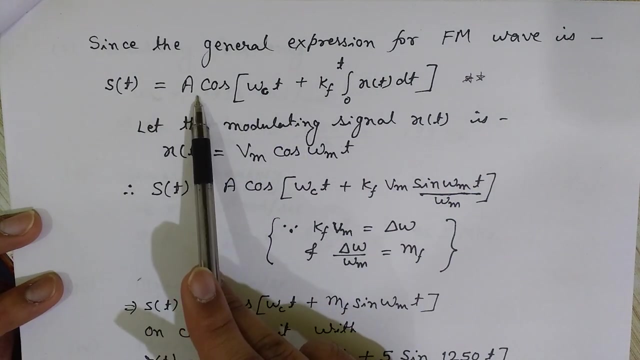 given by this equation: s, t is equals to s, t is fm. modulated wave is a cos of omega c, t plus kf, integral 0 to t, x, t, dt. You learn this thing but it is very important equation. Keep this in mind. So a is what, a is the maximum amplitude- Okay- Of this modulated wave and omega c is what. 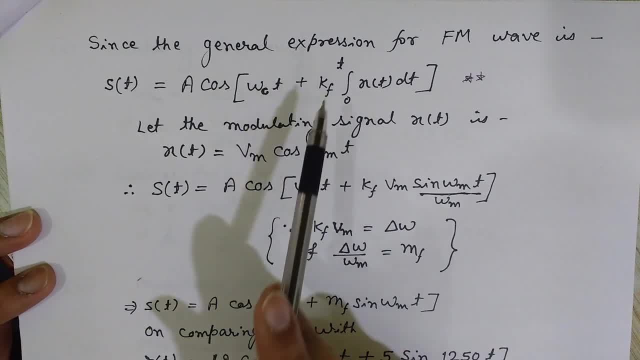 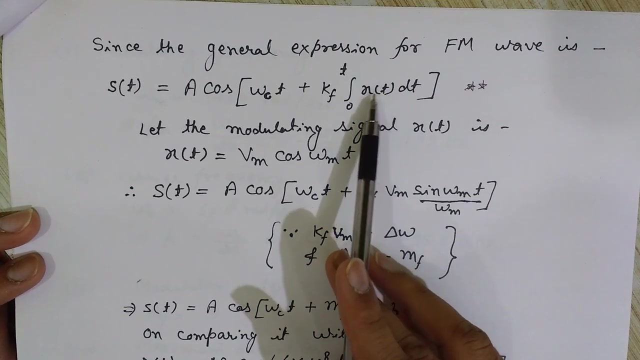 Omega c is the carrier. frequency, kf is what? kf is the proportionality constant and is also known as the frequency sensitivity. Frequency sensitivity of the wave is the frequency sensitivity of the wave. Now let's look at the modulator and x. t is the message signal, Since it can contain various 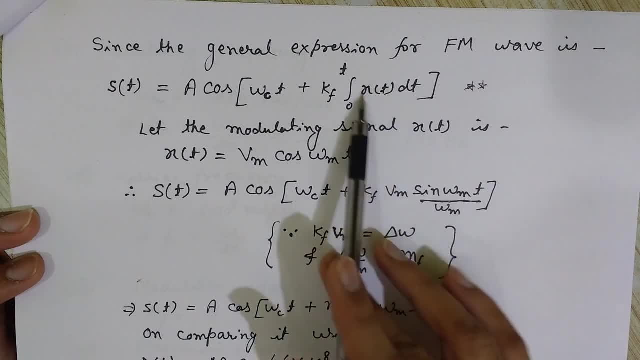 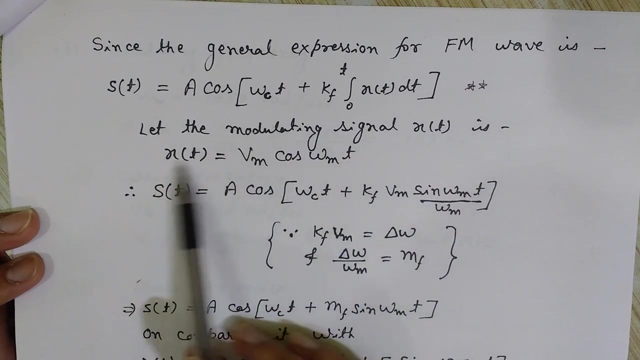 frequencies also, but, as in our question, it is a single tone, fm. it means it is containing only one type of frequency, not multiple frequencies. Now let the modulating signal: x, t is given by this. This is a single tone modulating signal, message signal, having vm is the maximum amplitude and 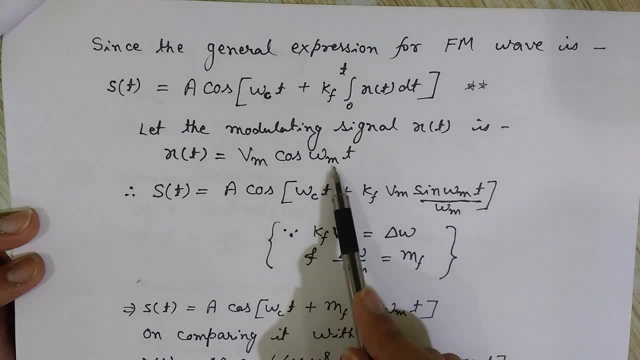 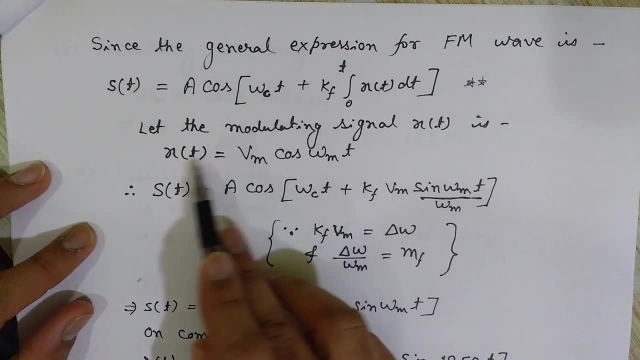 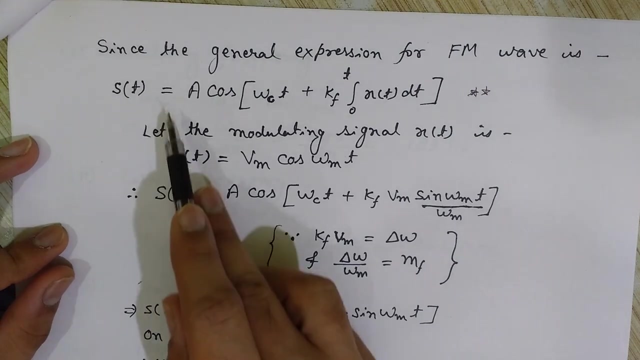 omega m is the maximum frequency present in the modulating signal. It has only one frequency component. It is a single tone message. Now here is the x t value. I will put this x t at this place. Okay, Now let's do this. s t is equals to. 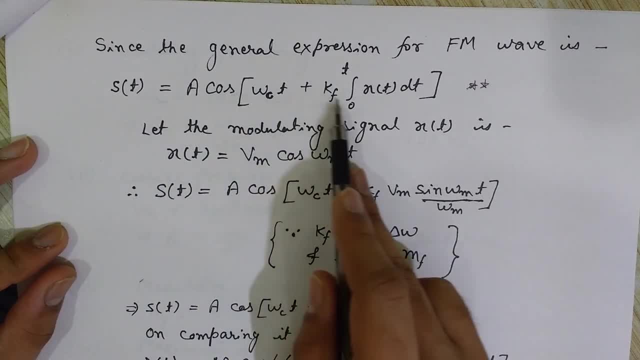 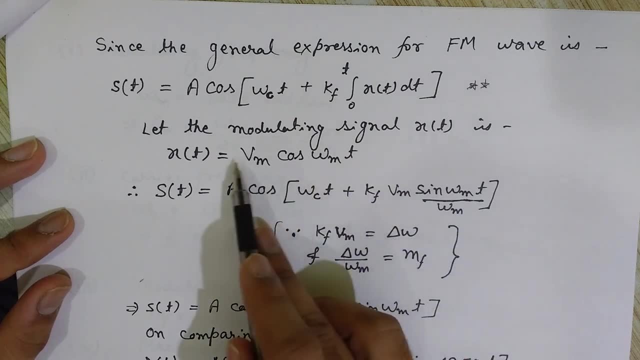 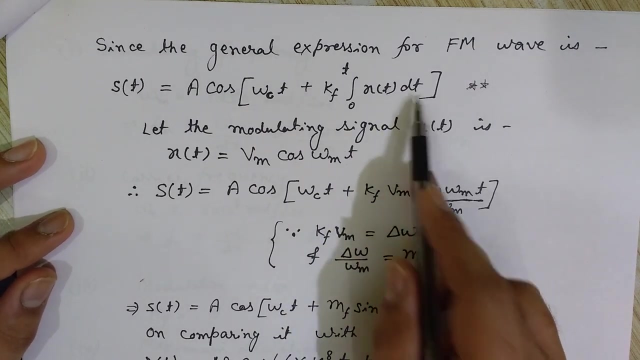 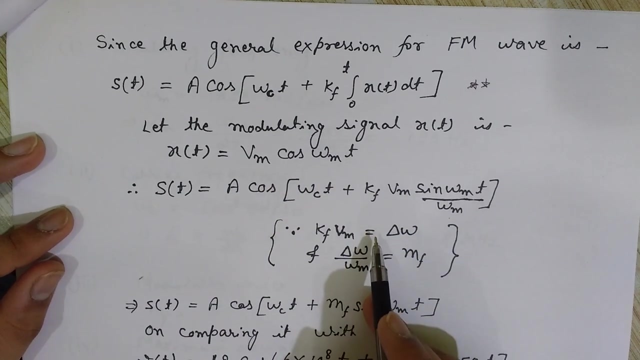 see this equation: a cos of okay, omega c, t plus kf. as it is Now, it is just the integration of x t here. So what is the integration of this? If I integrate this vm cos, omega m t with respect to, with respect to t, So it will be vm sin of omega m t by omega m. Now see here that this part kf into. 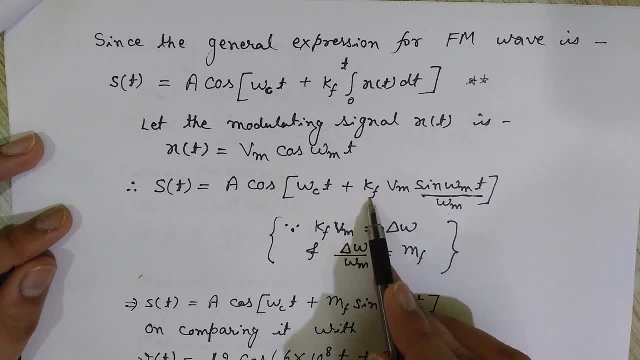 vm. Kf is what. Kf is the proportionality constant, also known as frequency sensitivity. Kf into vm is nothing but the delta omega. What is delta omega? It is the frequency deviation. Deviation of vm can be replaced by delta omega. So at this place I will write delta omega and in the 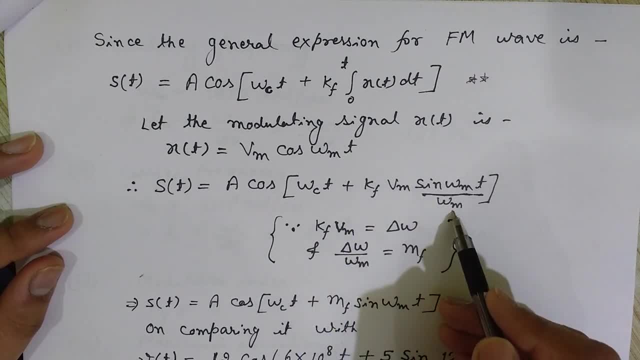 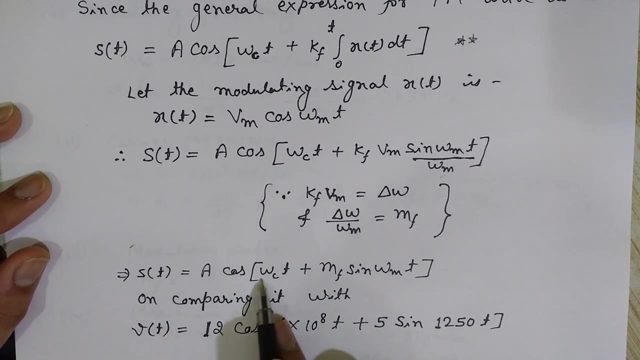 denominator. I have omega m, So it is delta omega divided by omega m, which can again be written as m f. So this, these three terms, this one, two and three, will convert to m f. Okay, I will write m f at this place. So s t is equals to a cos of omega c t. this omega c t plus this part is m f and 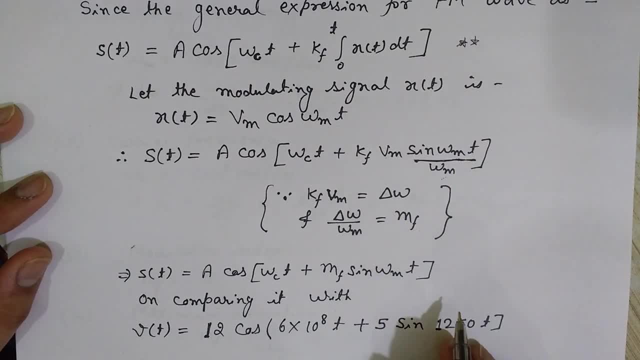 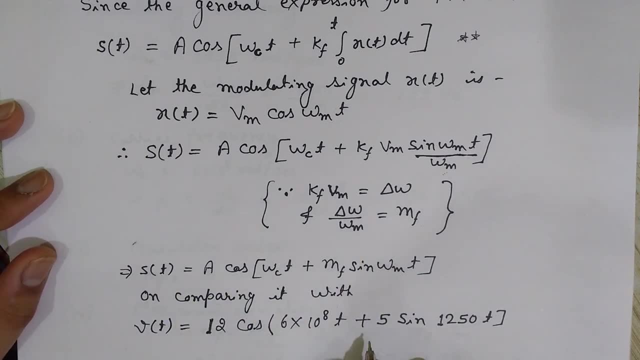 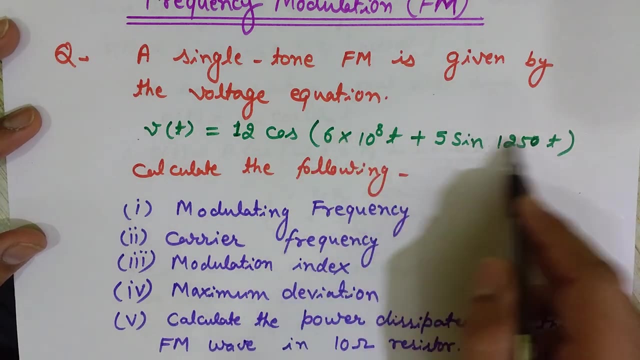 term is sin, omega, m, t. Okay, I think it is clear. Now I can easily compare it. compare this equation with the given equation, Our given equation. the question was this: Okay, This was the equation given, So let us write this equation again for comparison purpose. v t is equals to 12. 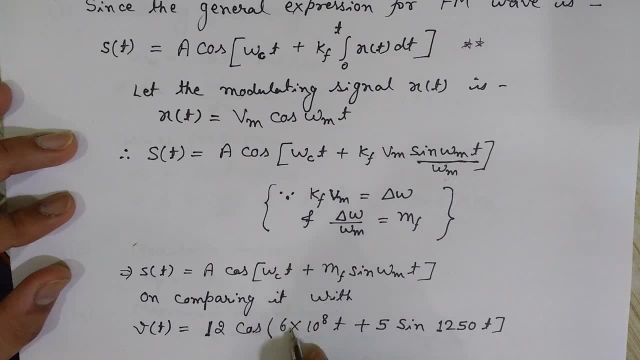 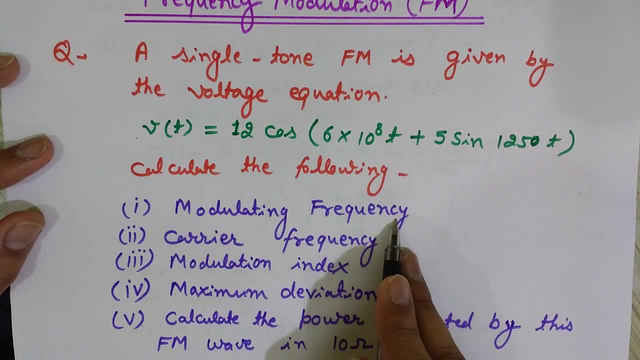 cos of this. Okay, You see this. Now we will compare these two equations and we will find. our first problem is to find the modulating frequency. Then we will find the carrier frequency in the second part. So, modulating frequency and carrier frequency, how can we find? 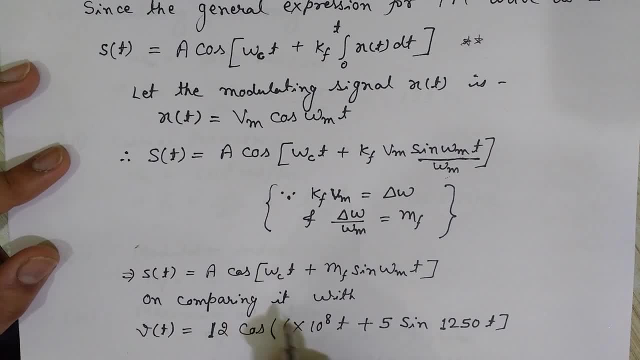 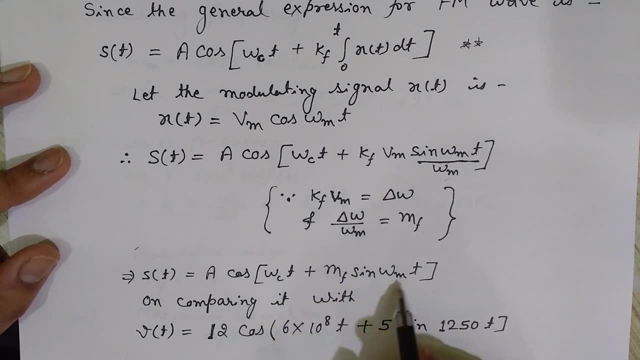 it by comparison: Modulating frequency. you see from this equation, modulating frequency is denoted by omega m. Okay, Where is omega m in this equation? The omega m is present at this place. sin of omega m, t. So you see here. sin of 1250 t. So omega m is. 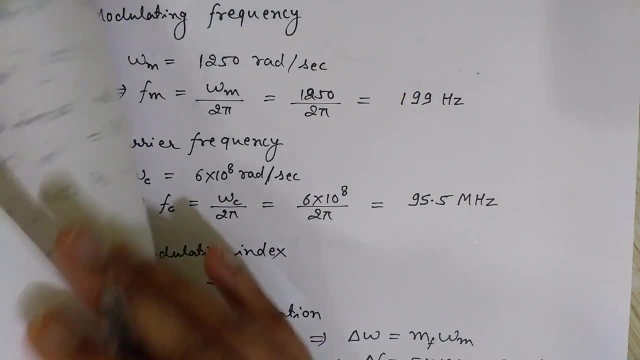 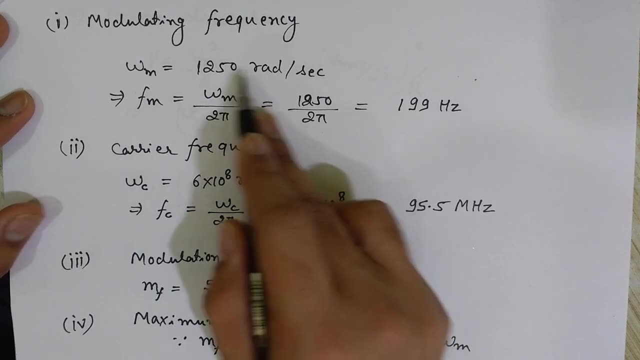 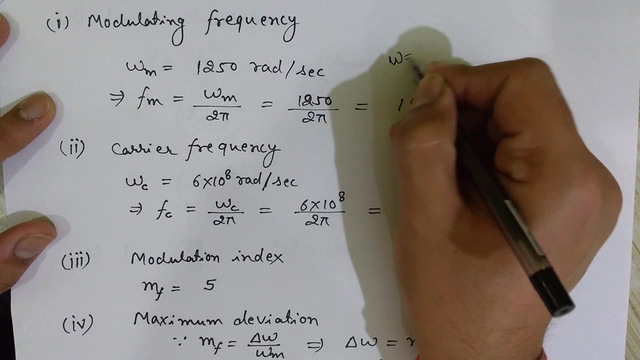 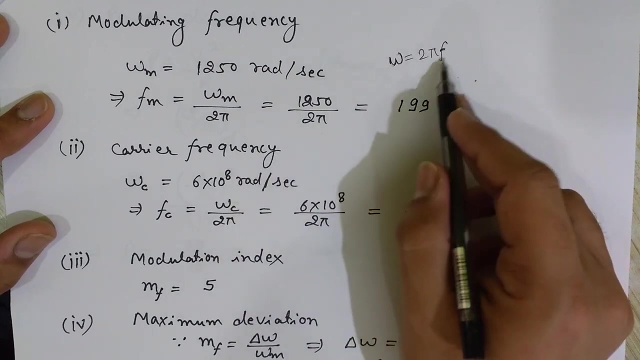 1250.. Okay, So this is our omega m. Okay, This is in. this is omega. it is in radians per second and I also know that what is omega? Omega is equals to 2 pi into frequency, So f will be omega divided by 2 pi. It will be in hertz. frequency is in hertz, So omega f. 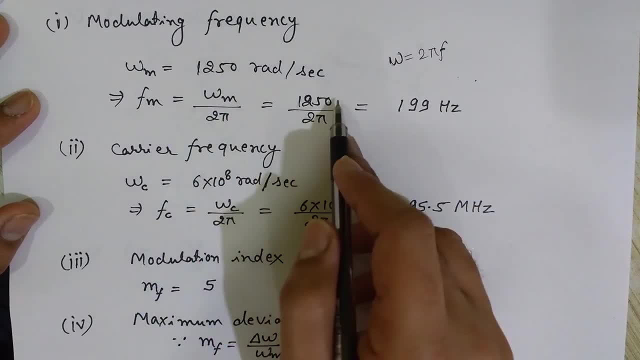 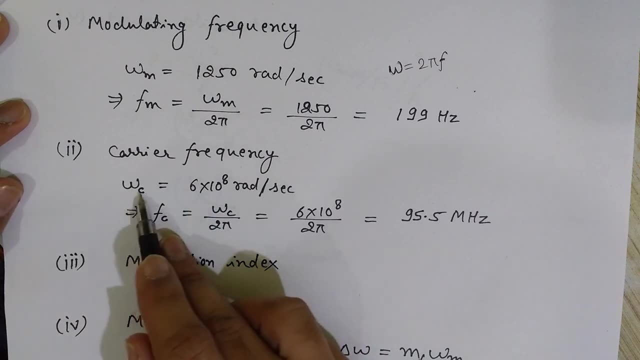 equals to omega by 2 pi. So omega m 1250 divided by 2 pi is 199 hertz. Okay, I got the modulating frequency. Now the carrier frequency. carrier frequency is denoted by omega c. Just by observation you. 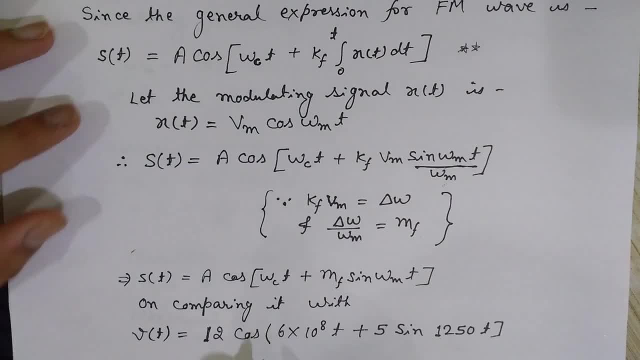 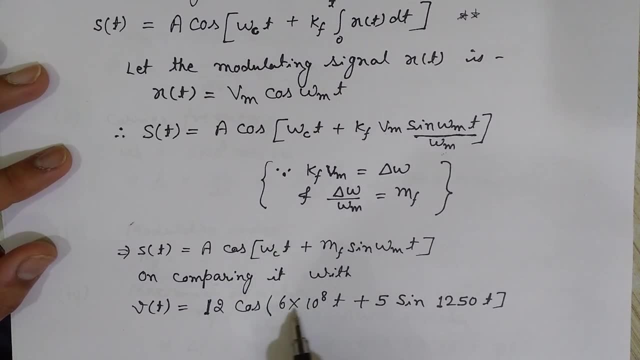 see comparison. omega c. where is omega c in this equation? Here is omega c. So this term after cos, before t, Okay, This term 6 into 10 to the power 8 is the omega c into t. So 6 into 10 to the power 8.. 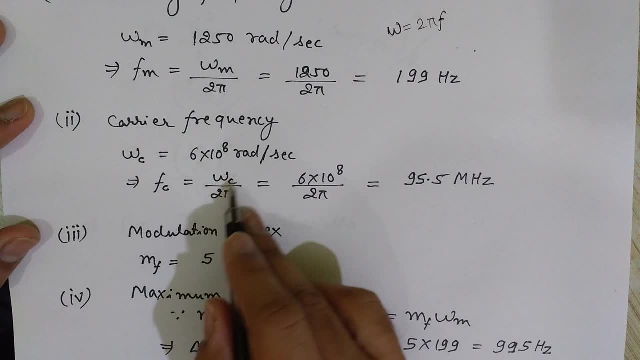 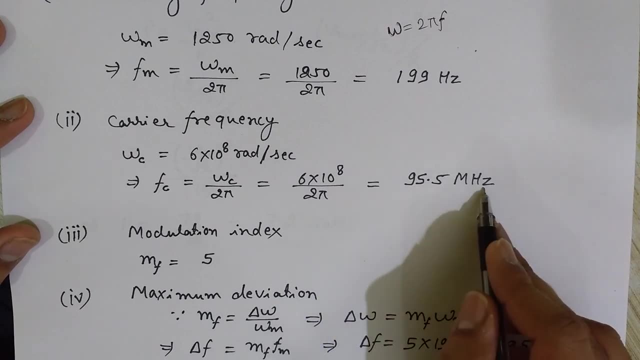 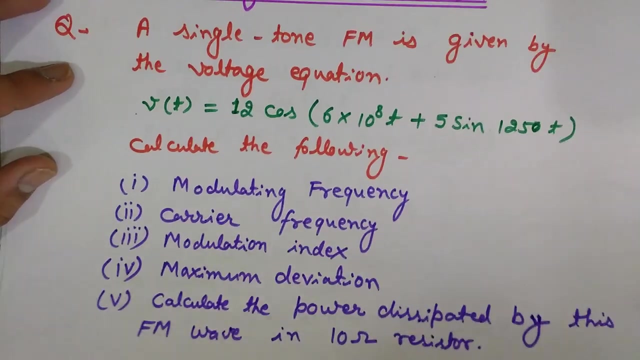 omega c, the carrier frequency. in the same way, i can divide it by 2 pi to find the carrier frequency. it is in radian per second and it is in 95.5 megahertz. it is in hertz. okay. the third thing is to find is modulation index. you see, here we want to calculate modulation index. and the fourth thing: 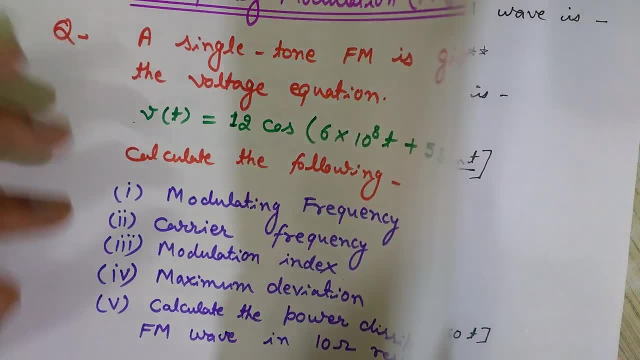 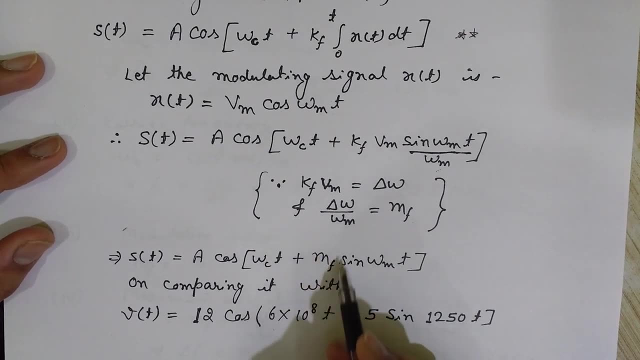 will be the maximum deviation. so modulation index and maximum deviation- now see modulation index- for fm is denoted by this mf modulation index, m for frequency modulated wave. so mf, mf is just before the sign. you see, this is so 5 is simply the modulation index at this place. 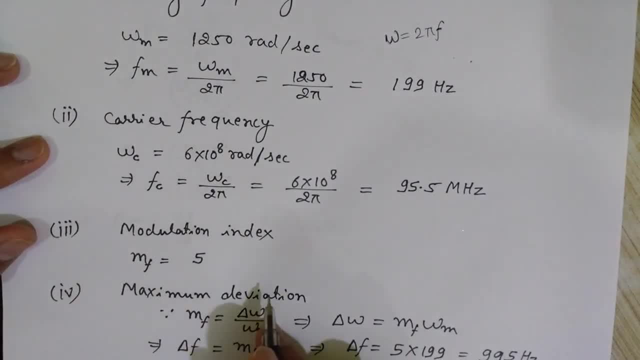 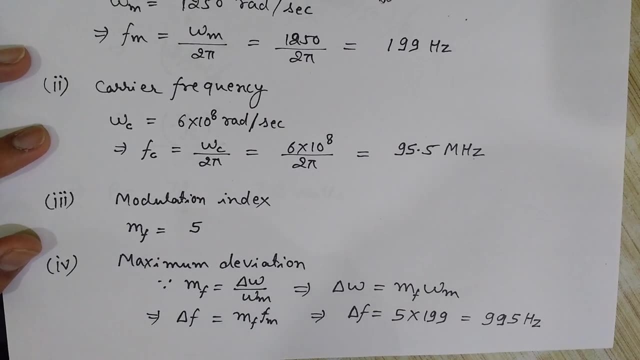 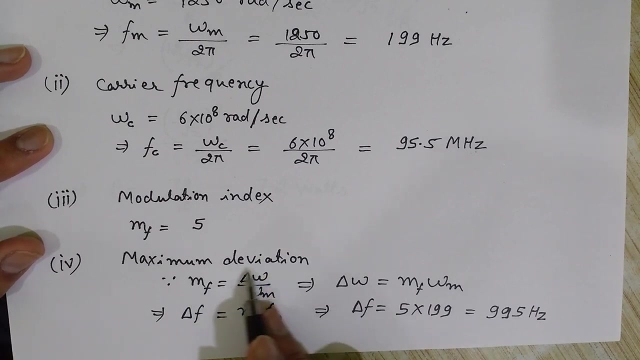 so modulation index is 5. it is very simple. and the maximum deviation? now see that maximum deviation. how to calculate maximum deviation? actually, the modulation index formula is synchronous omega by omega m. we can find the modulation index by dividing the frequency deviation by the omega m, the maximum frequency component present in the modulating signal. so delta omega will be from: 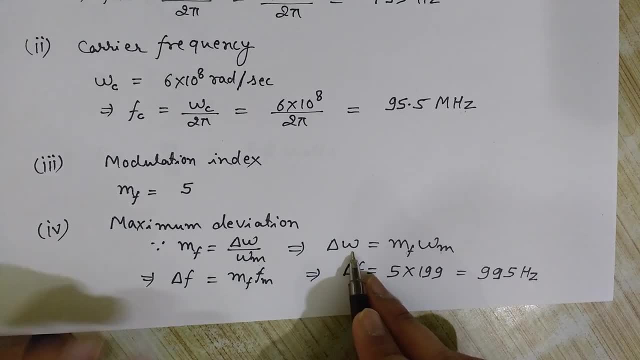 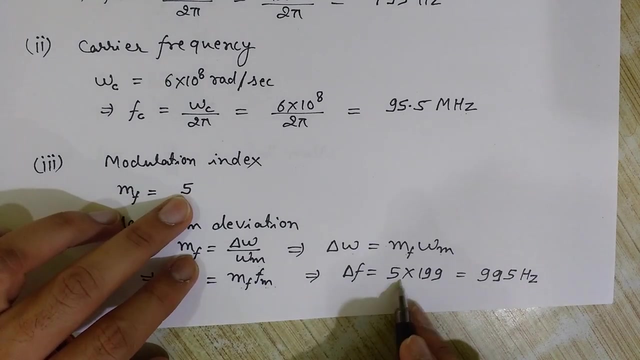 this mf into omega m. instead of delta omega, i can calculate delta f also and delta f will be mf. same and instead of omega m i will use is here fm. actually this can be easily converted to this by dividing both sides by 2 pi. so delta f is mf into fm. i know mf, mf is 5 and fm. fm is what fm is. 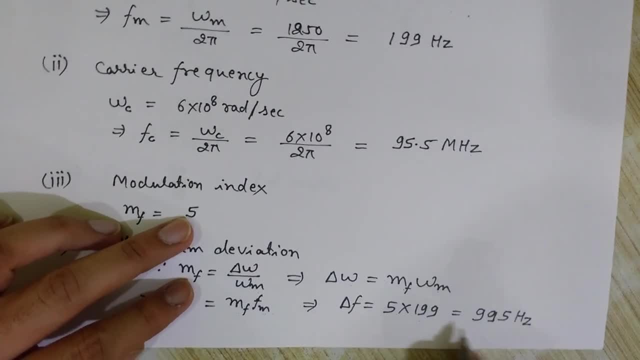 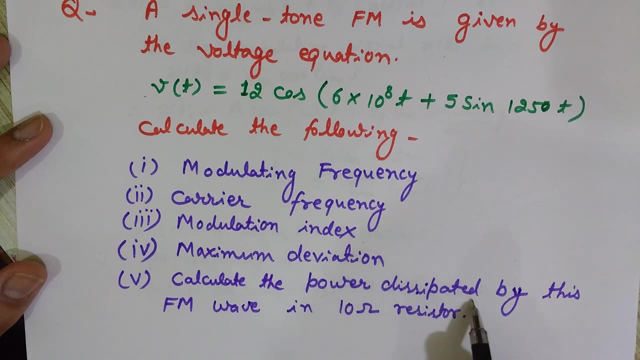 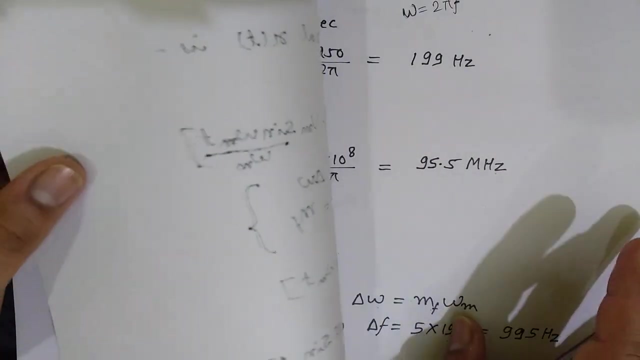 199 hertz, so 199 hertz, so 995. so this was the maximum deviation. now the last thing that i want to calculate is: the power dissipation is calculated by this fm wave in 10 ohm resistor. okay, dissipated power in the 10 ohm resistor: how? 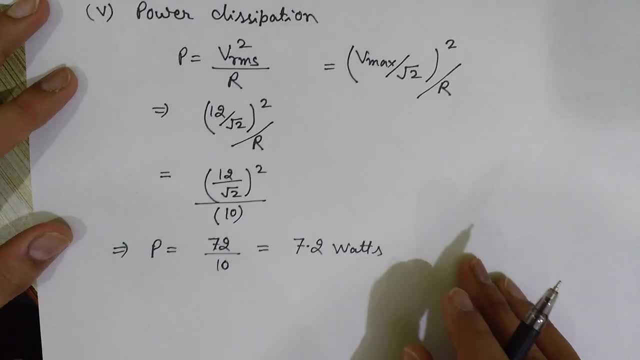 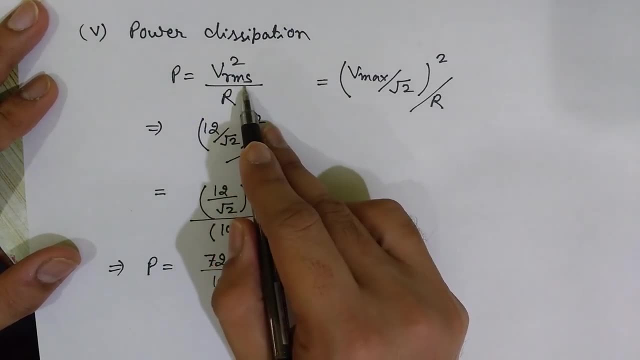 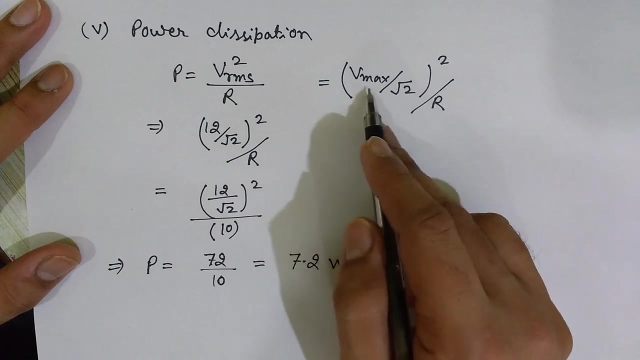 can i calculate it? since the power dissipation, the standard formula for power is what v rms square divided by r. okay, v rms rms is root, mean squared. okay, so v rms voltage and square divided by r, and formula for v rms is v max by root 2, if i have the 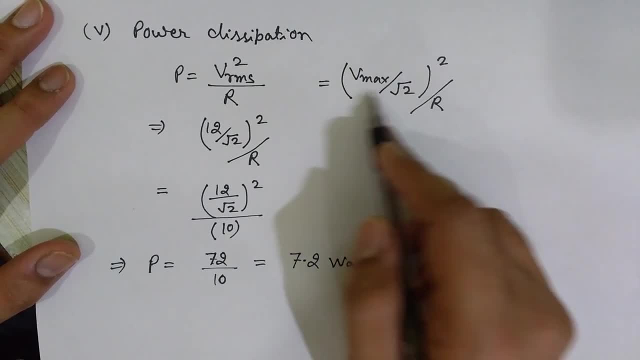 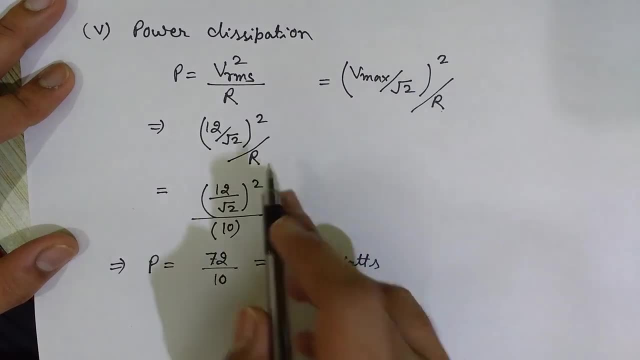 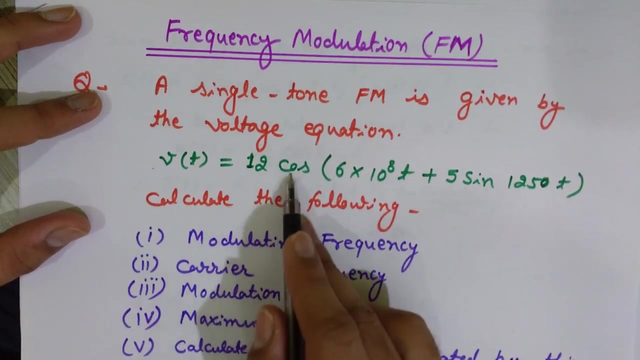 maximum value of amplitude and i, divided by root 2, i will get the rms value. so v rms is v naught or v max by root 2 square divided by r. what is v max? v max is from this equation v max. is this okay? 12?